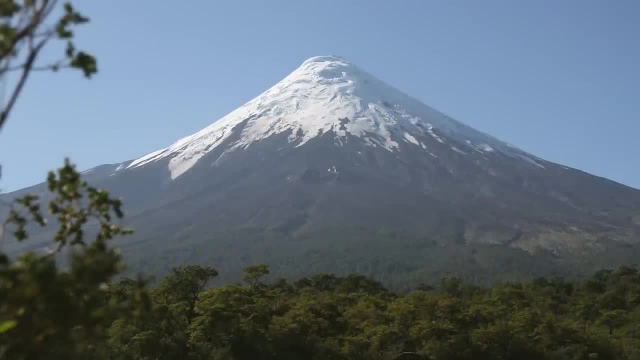 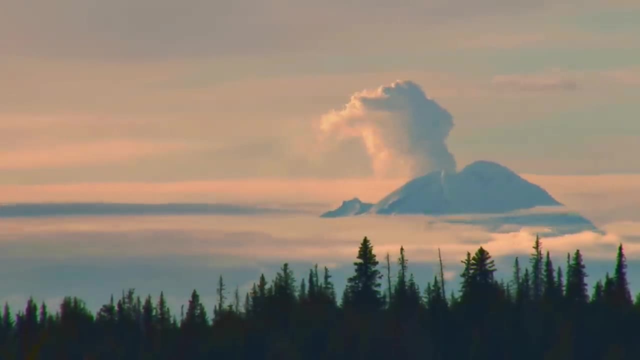 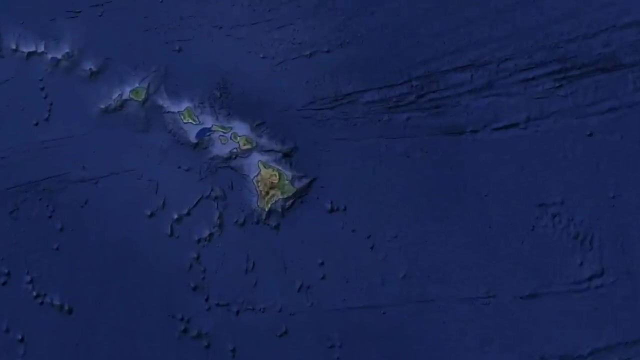 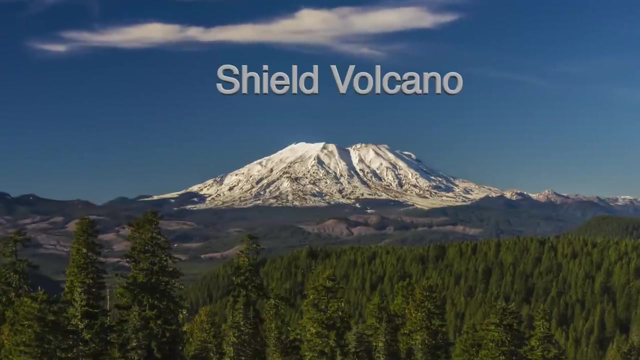 and may someday erupt, Or a volcano may be extinct, which means that it was once active but will probably never erupt again. Let's explore three types of volcanoes. Millions of years ago, the islands of Hawaii emerged from the sea, powered by erupting volcanoes. The formation of the islands of Hawaii are examples of shield. 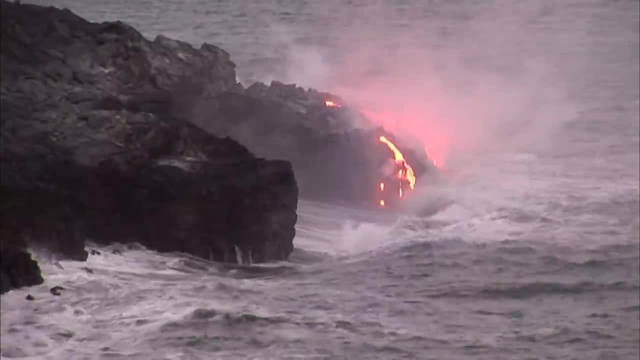 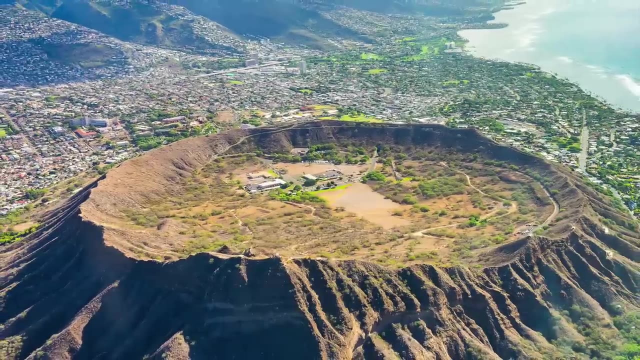 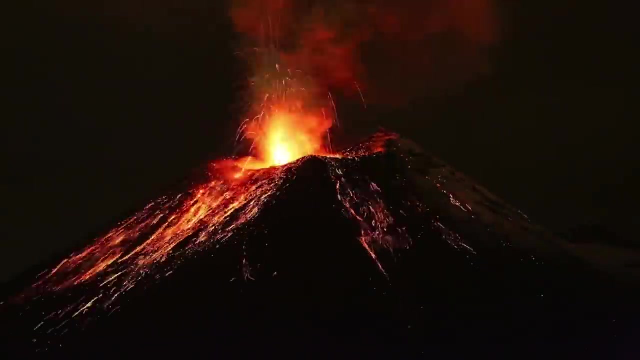 volcanoes. Some of these volcanoes are active and continue to erupt. Other volcanoes have been dormant for a million years. These volcanoes are massive in area and have gradual sloping sides. The eruptions are like fountains and lava flows are very liquid. The Loihe volcano, south of the. 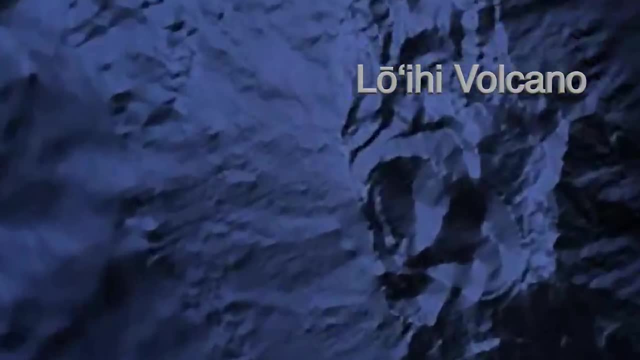 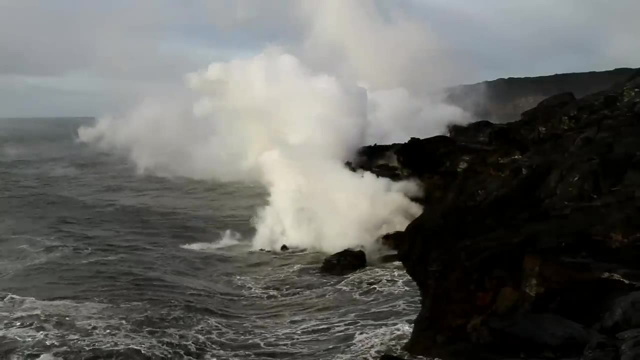 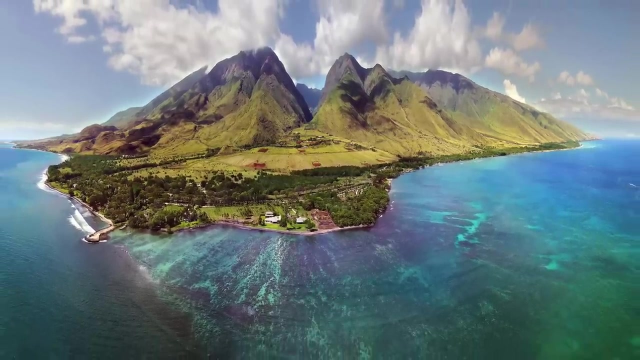 big island of Hawaii is one actively erupting volcano under the sea. Loihe is a seamount rising 10,000 feet from the floor of the Pacific Ocean And as it continues to erupt molten lava, it one day will become an island all its own in about 100,000 years. Shield volcanoes are not as explosive. 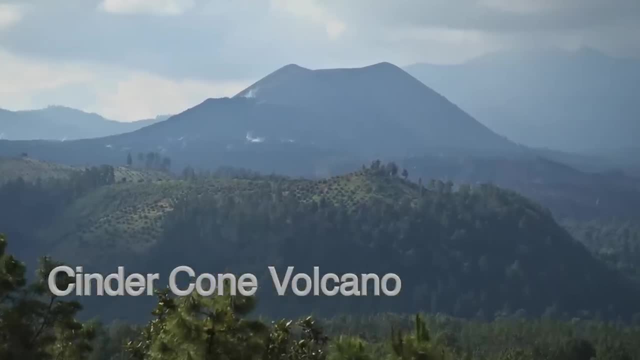 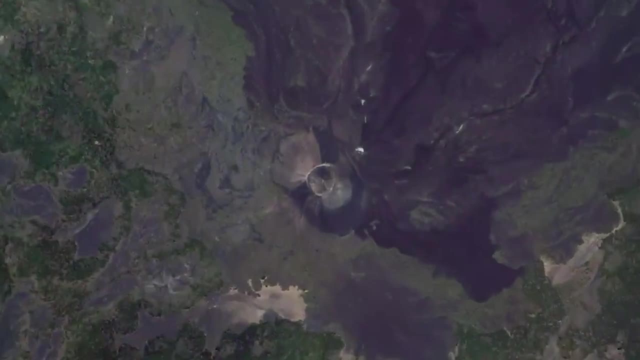 as shield volcanoes. They are not as explosive as shield volcanoes. They are not as explosive as cinder cone volcanoes. A cinder cone volcano has straight, steep sides. In 1943, Senor Pulido was working in his cornfield near the village of Paricotin, Mexico. Pulido tells the story that 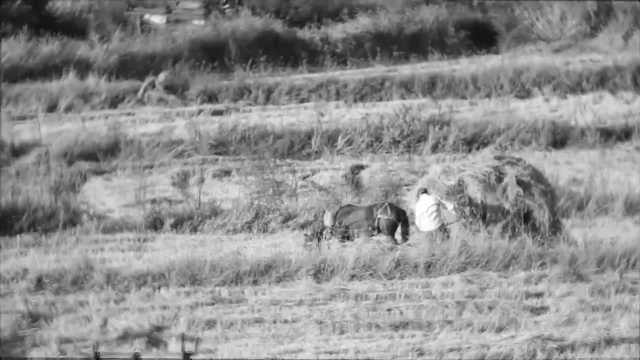 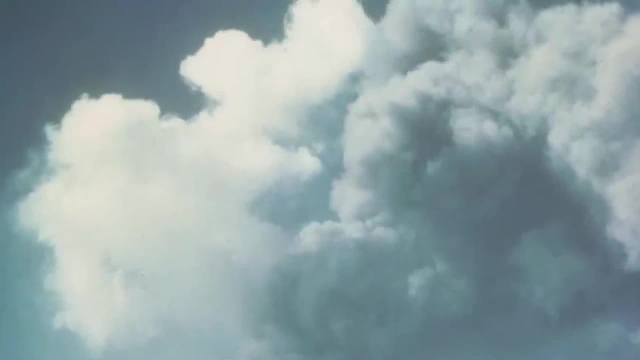 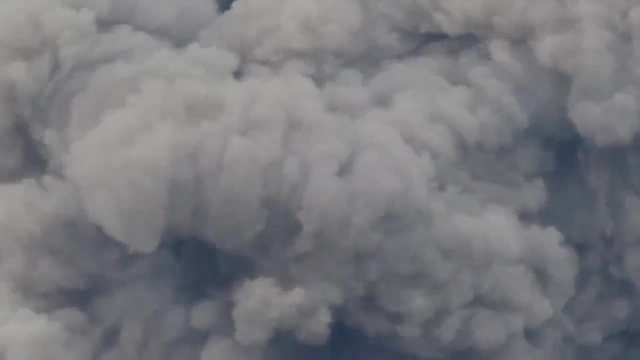 as he and his family were working in the field that the earth began to tremble and shake And right before his very eyes, the ground swelled to over six feet, A fissure opened and gray ash and smoke poured into the air And the sound of a terrible hiss and the horrible smell of sulfur. 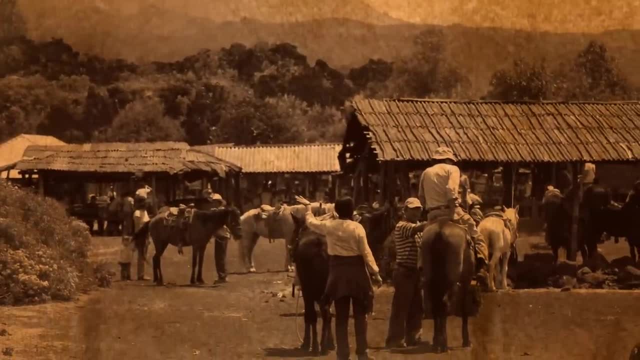 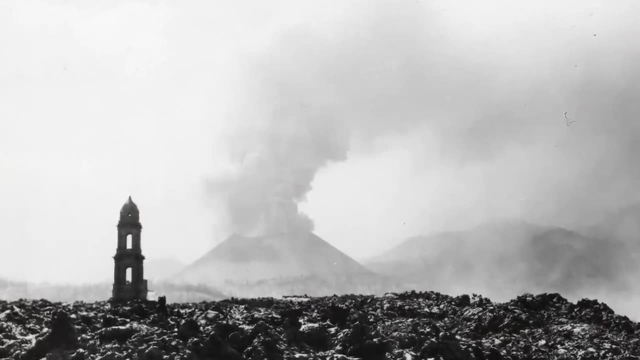 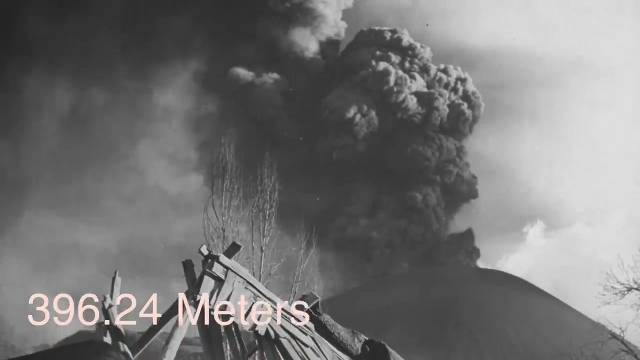 Through the thick smoke, Pulido could not find his family. He went back to the village and discovered they had arrived there safe and sound. Through the days and weeks and years that followed, the volcano would continue to grow to over 1,300 feet high, or 396.24 meters, spewing. 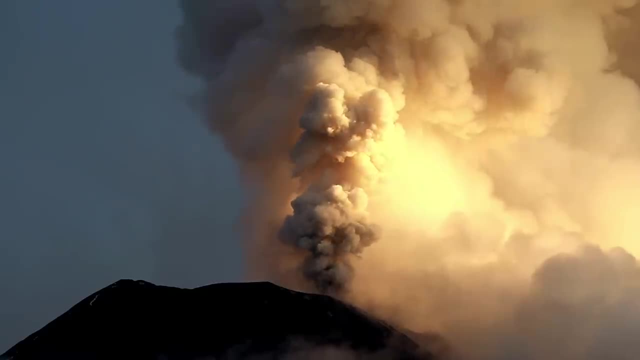 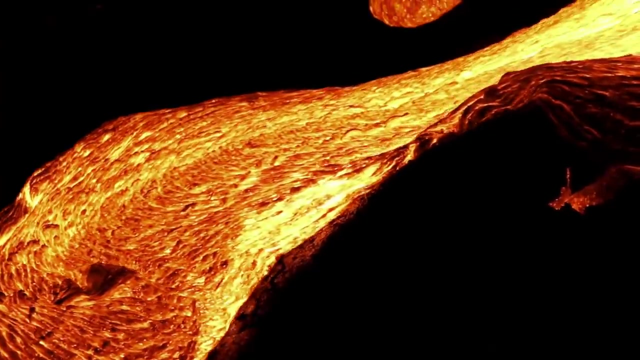 hot smoke and ash into the air Anyone who had to be evacuated and find another home, as thick, slow-moving lava would advance to the villages of Paracutin and San Juan, which were destroyed. Can you imagine how awful that would be? 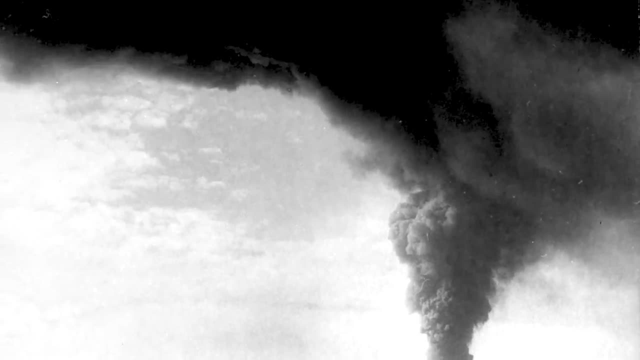 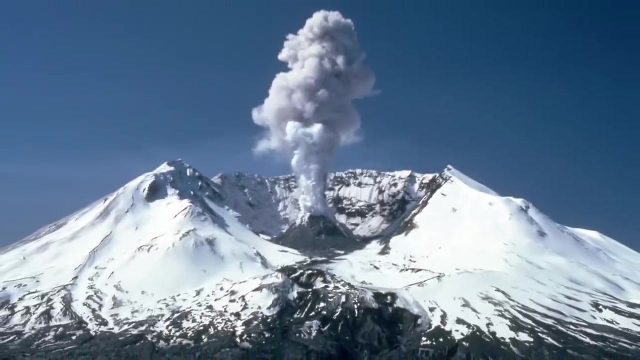 The Paracutin volcano has been very important to scientists, as they have seen the birth and rise of a volcano and watch it become dormant. And though a cinder cone volcano may be terrible, it is no match for the spectacle of a volcano where it is. 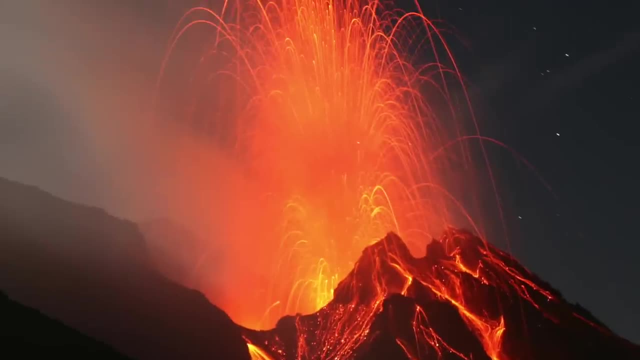 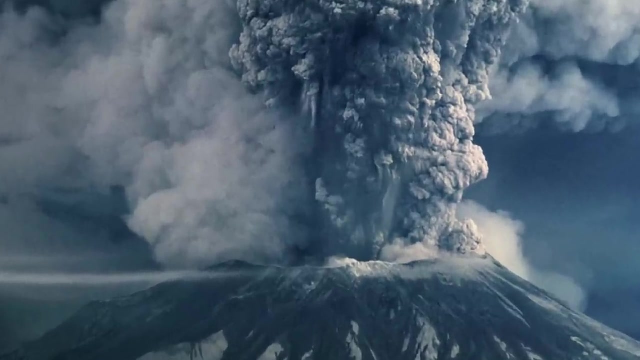 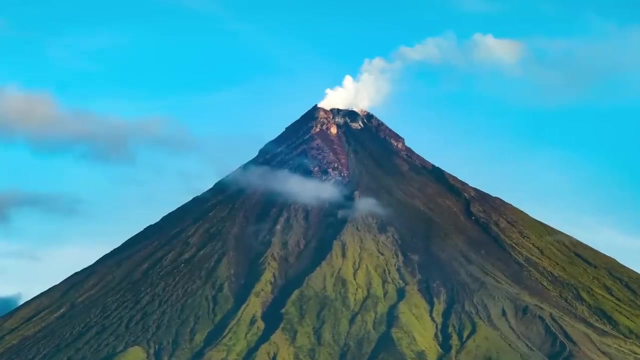 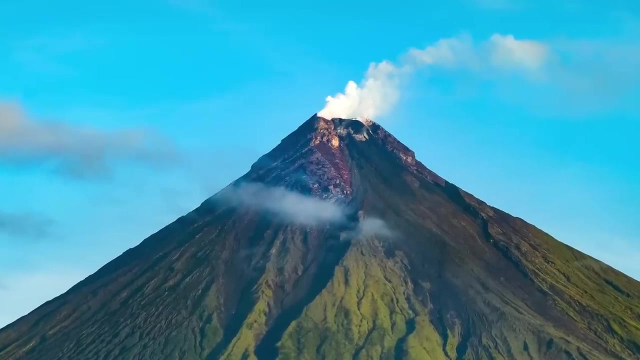 of a volcano which can be far more powerful, far more terrible, far more frightening and more explosive. Of course we are talking about the Stratovolcano. A stratovolcano is characterized by gentle lower slopes gradually increasing to steep upper slopes. They are constructed of layers of hardened 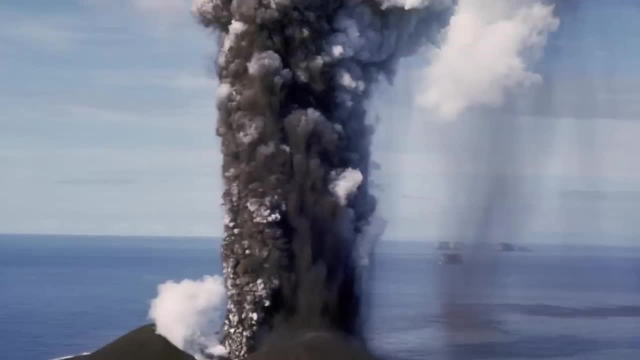 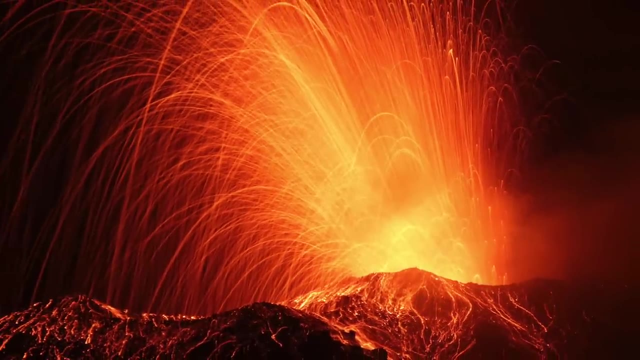 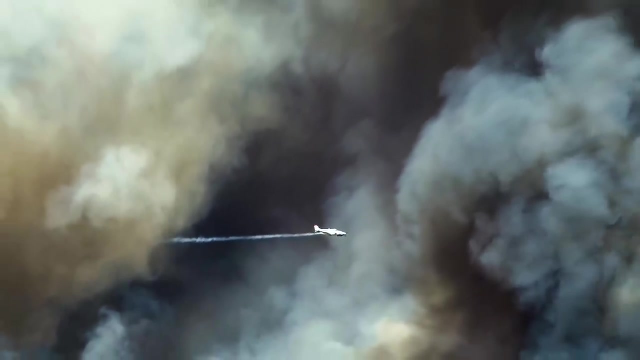 lava and volcanic ash and pumice. Stratovolcanoes are known to have violent eruptions expelling fiery lava fragments through the air like bombs. Toxic gases fill the air and massive plumes of ash clouds carry vast distances, making aviation travel impossible. These volcanoes are dangerous and deadly, and 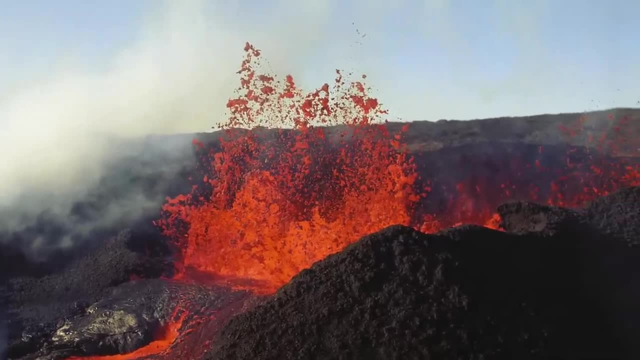 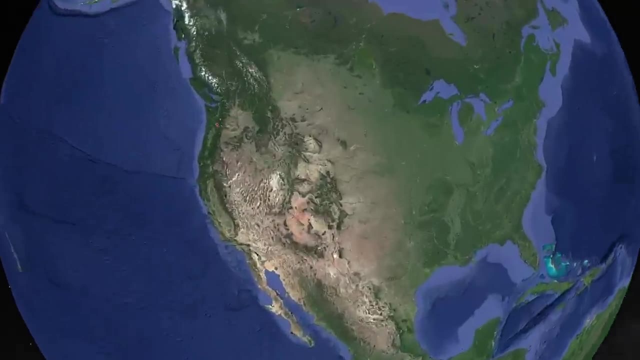 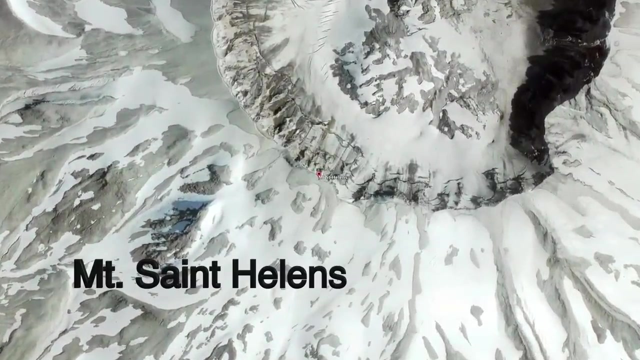 though lava from these volcanoes flow slowly, it covers and burns and destroys everything in its path. In the Cascade Mountain Range of Southwest Washington State, there rises many beautiful snow-covered peaks. Some of them are volcanoes. One of these volcanic mounts is known as Mount St. 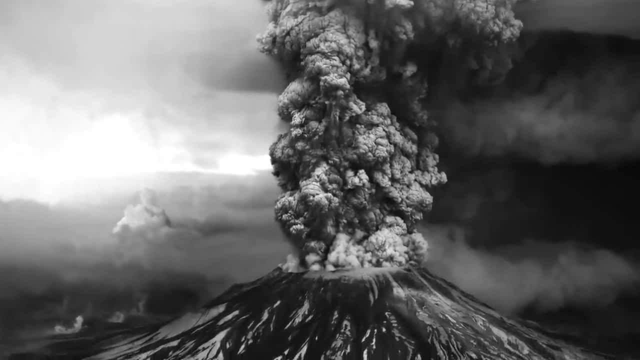 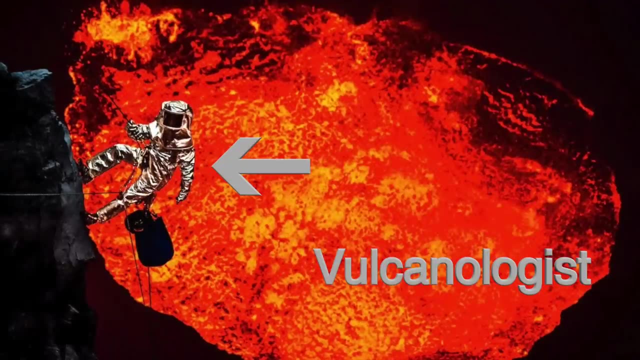 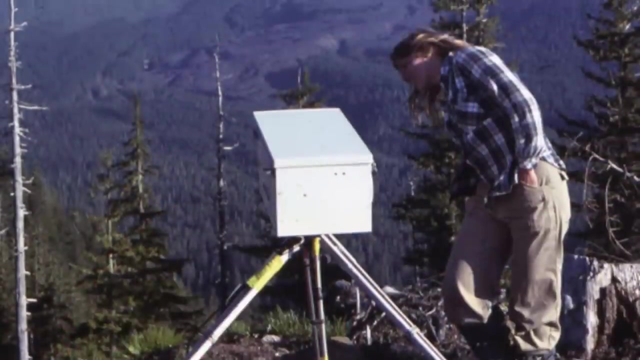 Helens. It was no secret that Mount St Helens had been an active volcano for hundreds, maybe thousands of years, and volcanologists- scientists who study volcanoes- had been studying St Helens with their equipment, watching and waiting for another, perhaps major, eruption. It was possible. 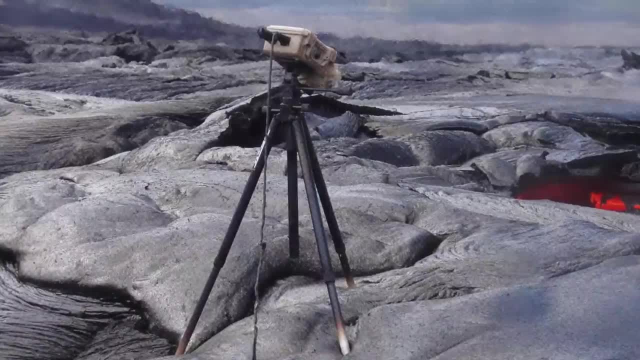 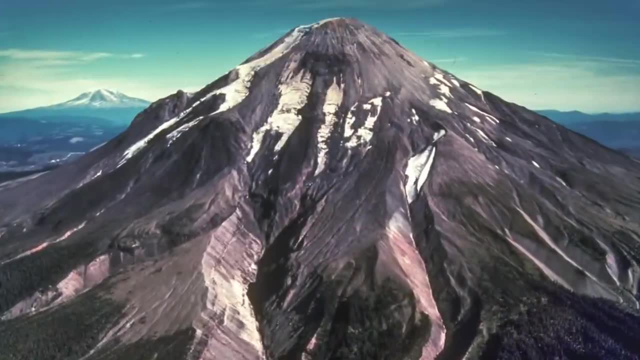 that St Helens would not erupt in their lifetime. Even with fancy equipment, these things are difficult to predict. Then came the spring of 1980. For months, tremors and earthquakes shook the ground On the north face of Mount St Helens a 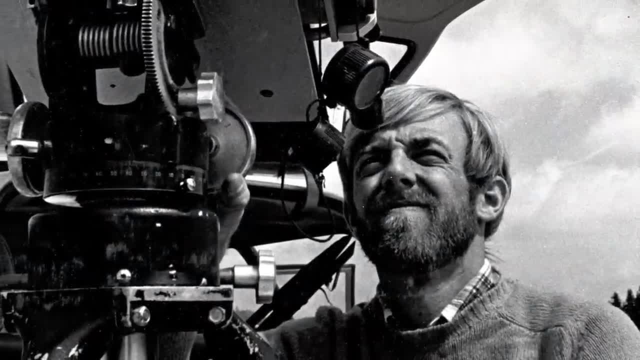 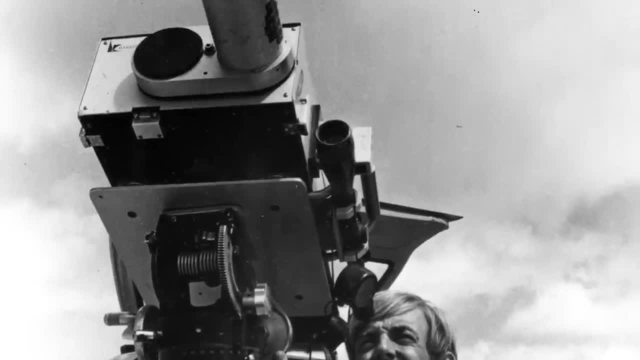 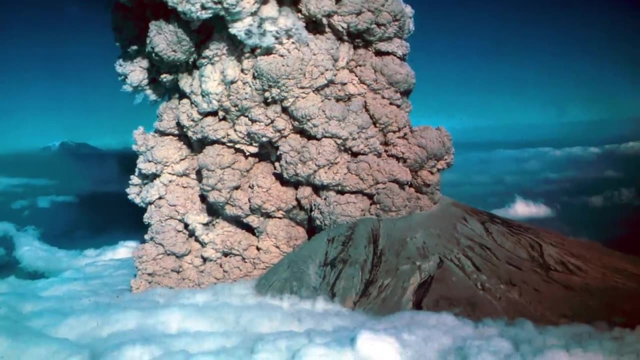 bulge began to form. Volcanologist David A Johnston was watching and measuring the growth of the bulge with his lasers. On May 18 1980, David called out over the radio: This is it, This is it. The caldera blew with supersonic fury Everything in the path of.